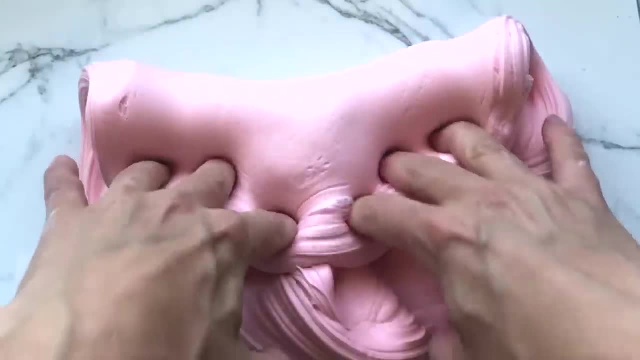 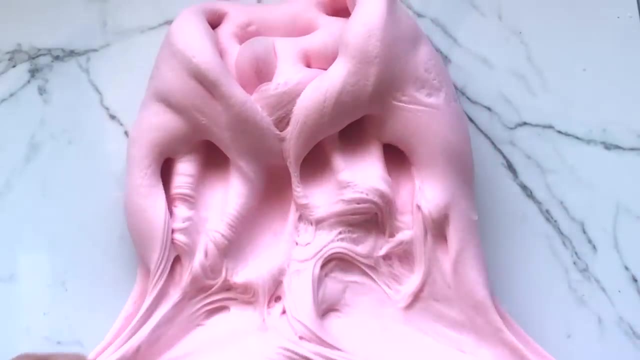 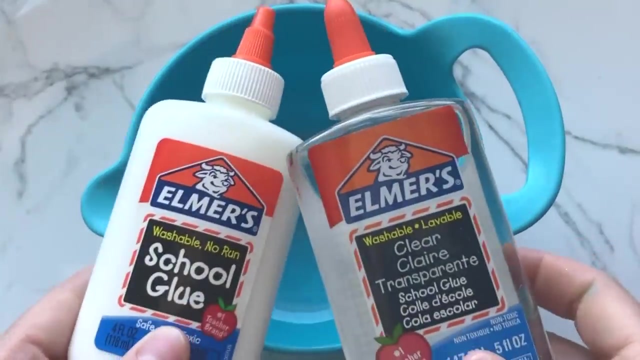 playmaker. welcome to my channel. consider hitting that like button if you found this video to be helpful and subscribe for more videos like this one. let's just jump right into the video and get started. all right, the first thing you are going to need is some Elmer's school glue. 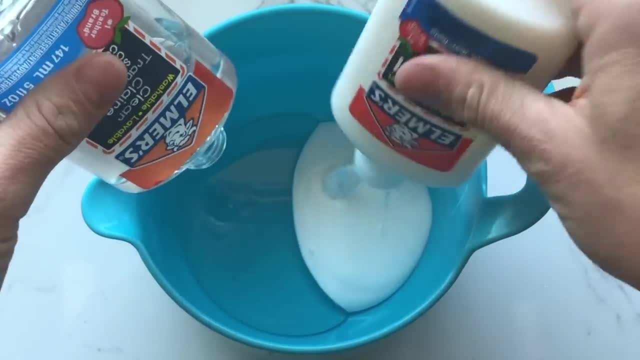 white and clear, so I'm adding that to my bowl. I like combining both glues to make this slime, but if you only have one or the other, you can use a little bit of glue. if you don't have one, you can use a little bit of glue. 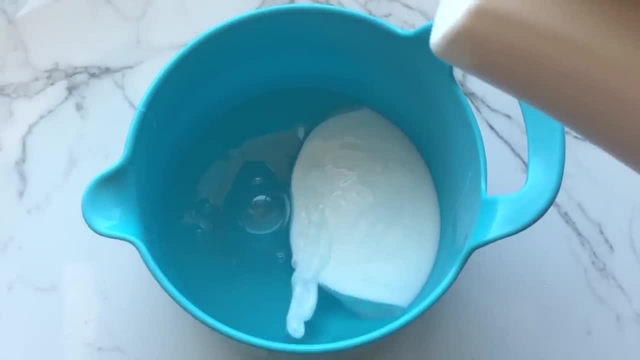 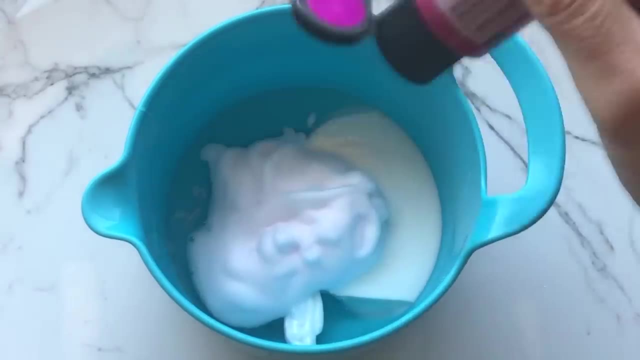 you can use that and it will turn out just fine. add a few pumps of lotion, add a few pumps of foam soap, and then you just want to either mix it up or add your coloring. you could use food dye, paint, whatever kind of coloring you like. mix. 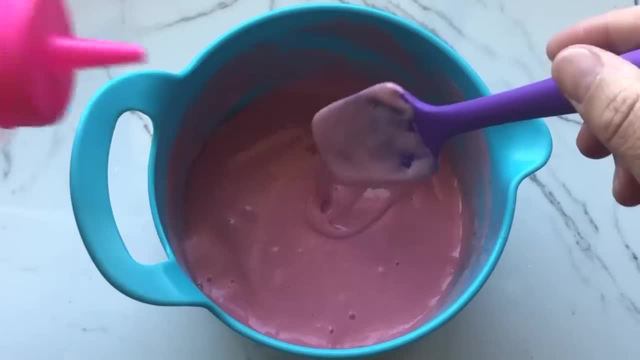 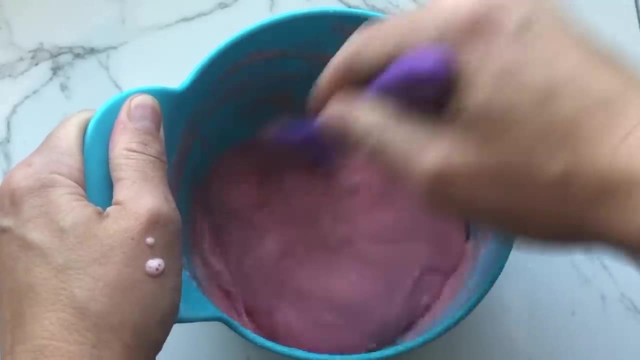 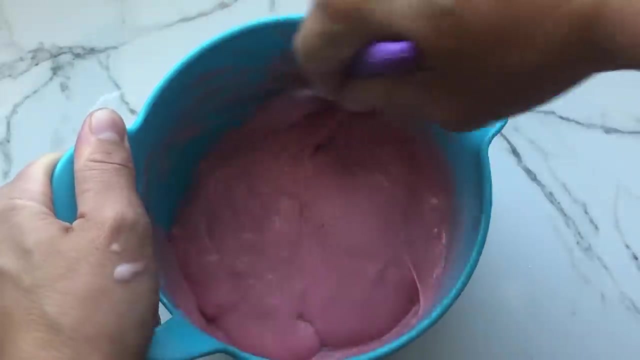 that all up and get ready for the activation. so once it's all mixed up, you're going to start activating. I'm using one teaspoon of borax dissolved in one cup of water. it's kind of my preferred method of activation for most of my slimes. so you want your slime to be not so sticky. 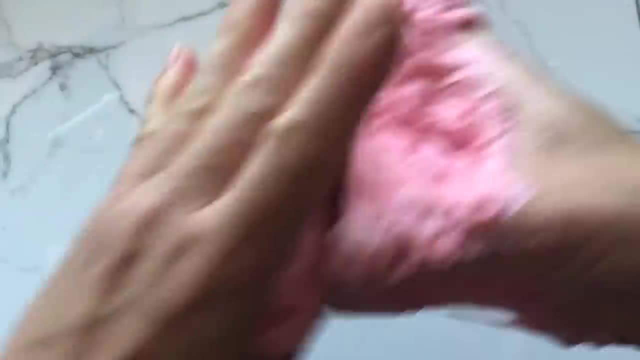 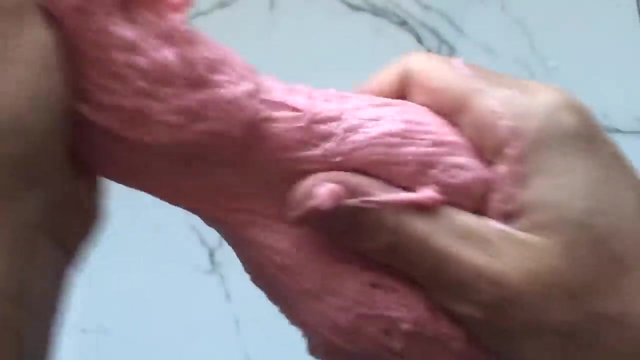 this is kind of where I'm at right now. I'm not going to add any more activator at this point. I'm just going to work it with my hands and it should eventually come together. a lot of people make the mistake of adding more activator at this. 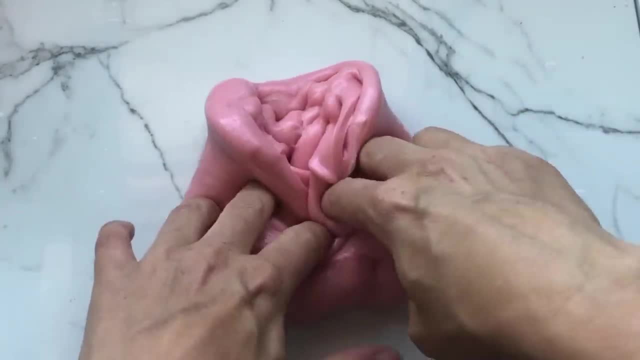 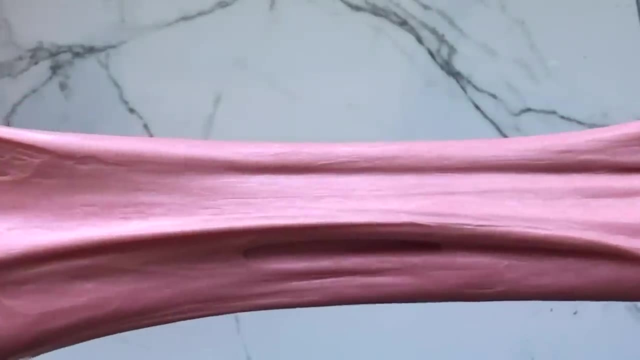 stage and you end up with a super stiff slime, and that's not what you want. now you can tell that this slime is not super, super stretchy, but it's stretchy enough because once we add it to the clay it will become stretchier. I like using the kawaii slime, a company 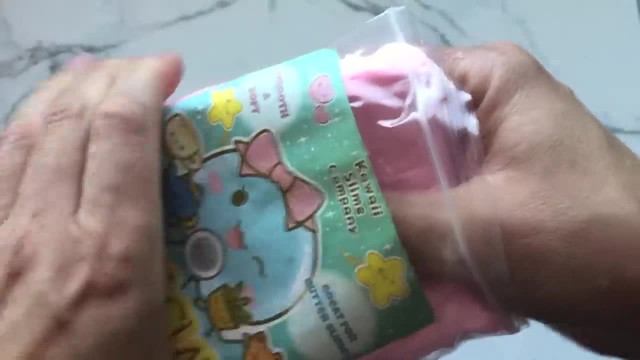 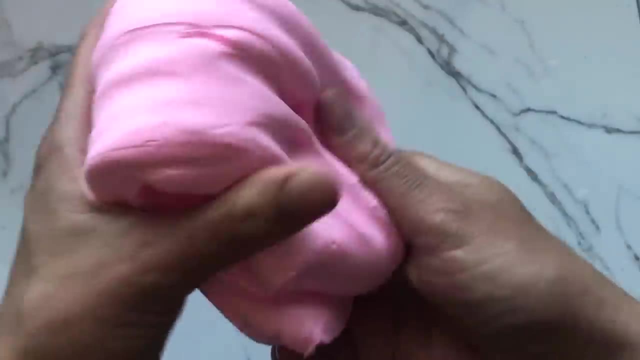 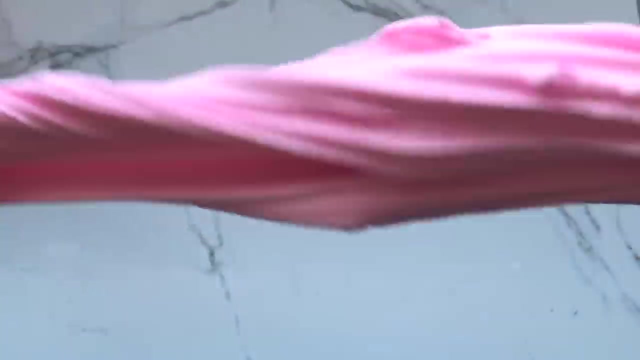 clay for my sizzly fluffy inflatable butter slimes. her clay is kind of like a slime already by itself. you can see how nice it stretches and really if you wanted to turn it into a slime, you can just add very little clear slime or very little white slime, and it will. it would be amazing, but I'm going to add a bunch. 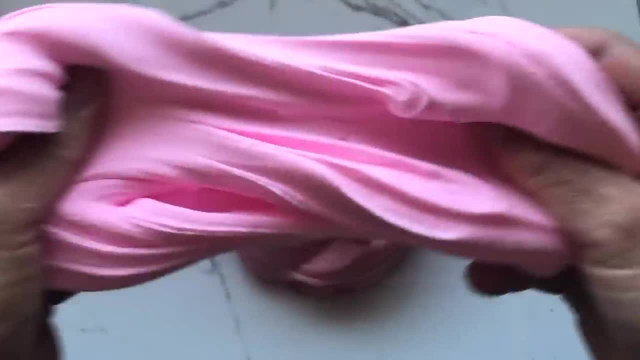 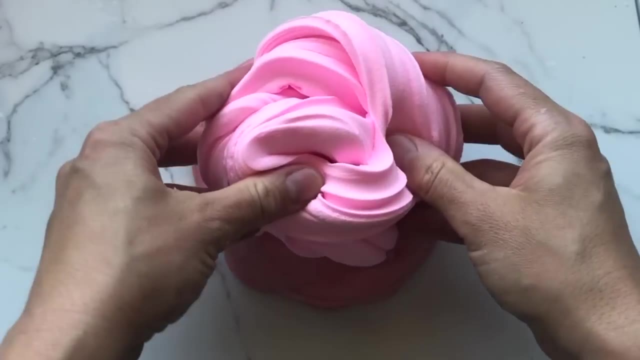 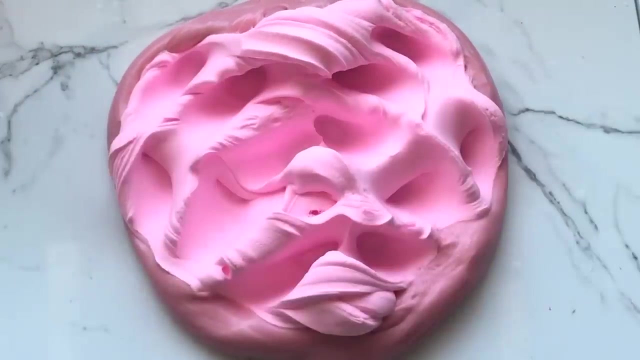 of slime to it. So I put my slime on the bottom and then I'm going to put this clay on top and then press it in, So you can kind of hear a little sizzle already at this point. It's going to be amazing when it's finished.